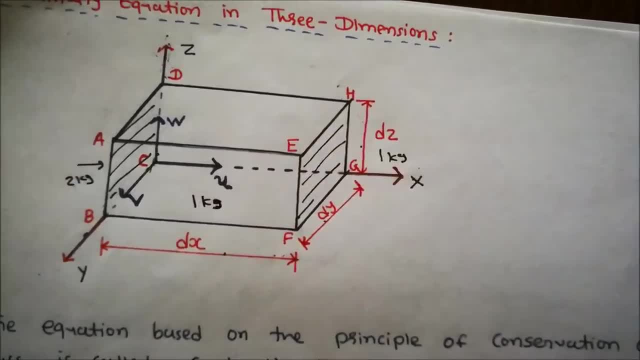 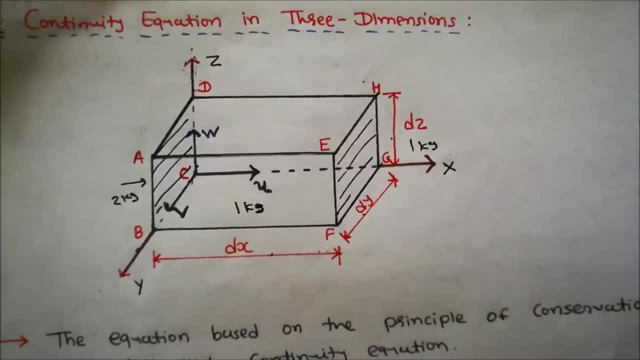 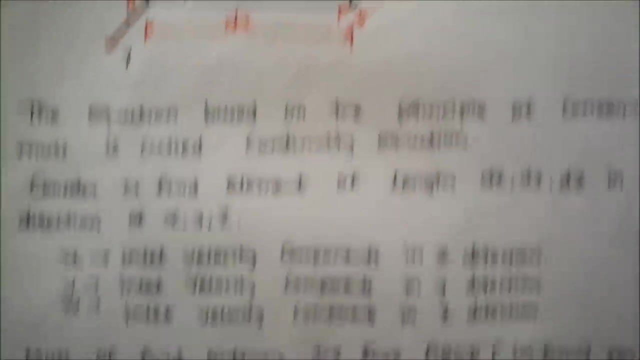 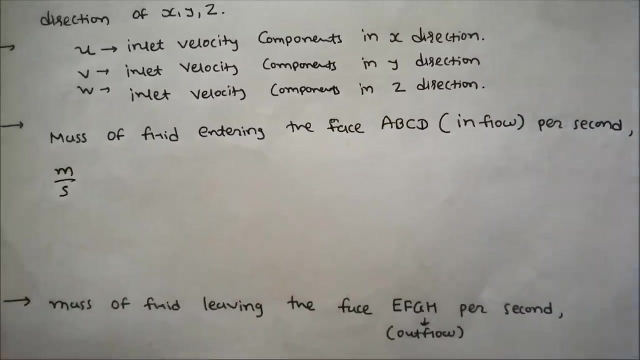 rate of increase of mass in the in mass in x direction, that is mass through abcd minus mass through efgh. so first we find mass of fluid entering the face abcd. so we find mass of fluid entering the face abcd per second, so mass per second. so what is the meaning of mass density? 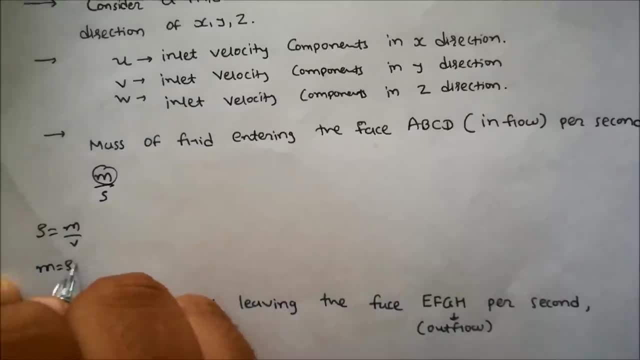 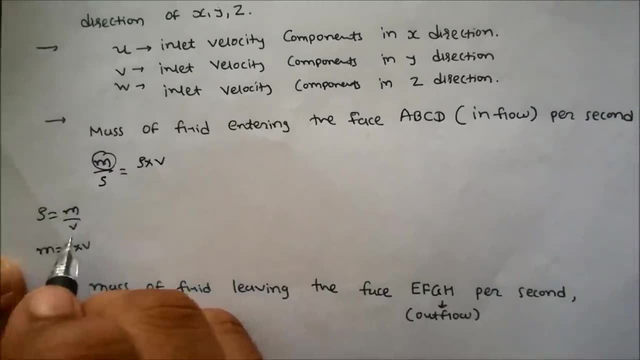 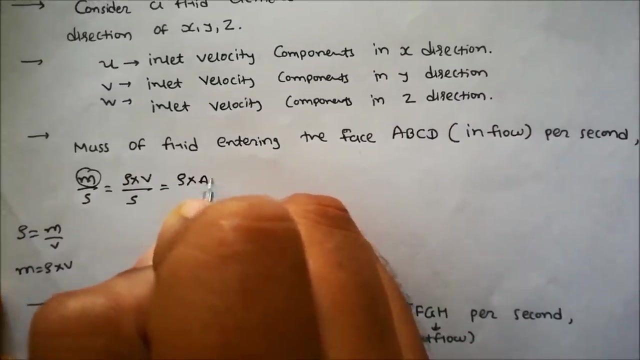 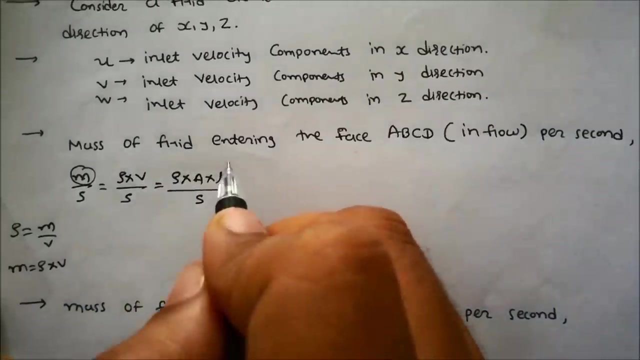 means mass per unit volume. so mass is equal to density multiply volume. so in place of mass we write density multiply volume, divide by second. so what is the meaning of volume? volume means area into length, so divided by second. so length per unit time is known as a velocity. distance per unit time is known as a velocity. 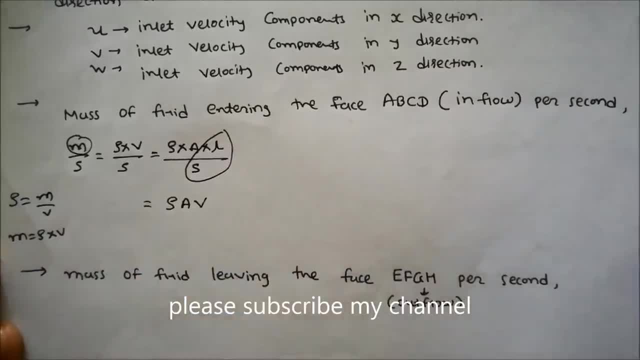 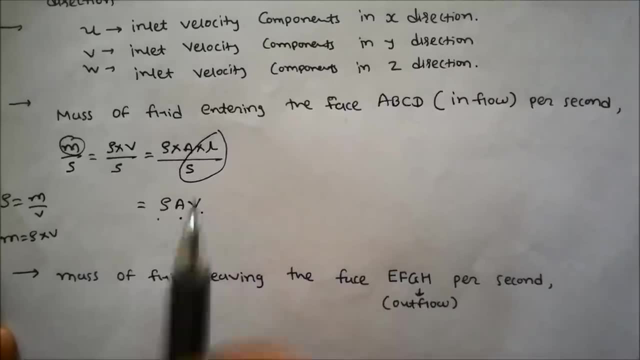 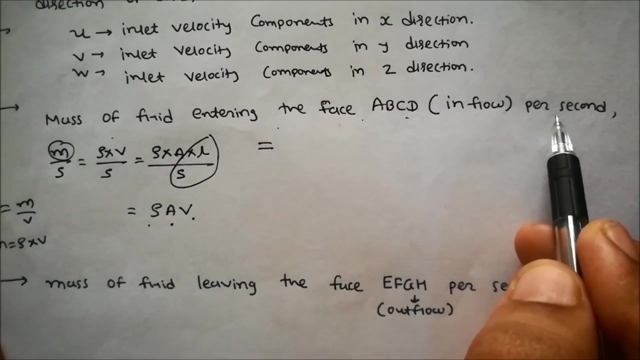 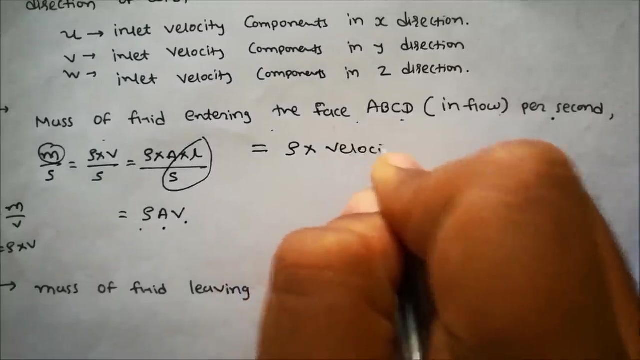 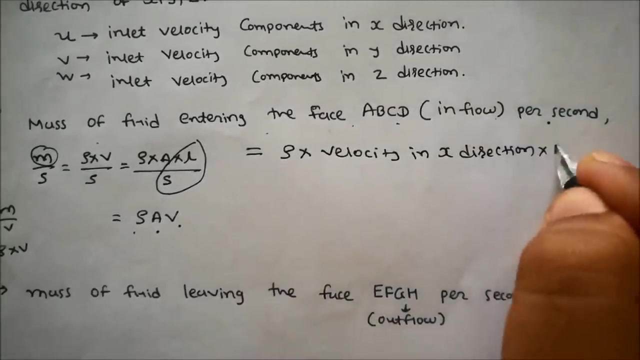 so we write rho, a, v. rho means density, a means area of abcd and v means velocity in x direction. so we can write mass of fluid entering the face. abcd per second is equal to rho multiply velocity in x direction. velocity in x direction multiply area of abcd. again, I repeat, 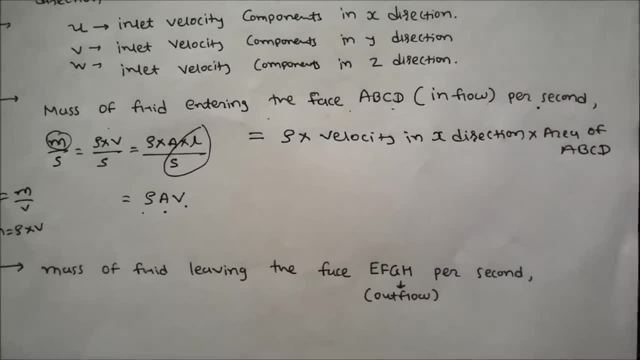 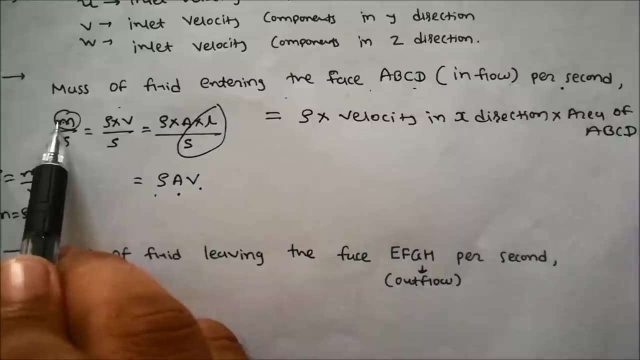 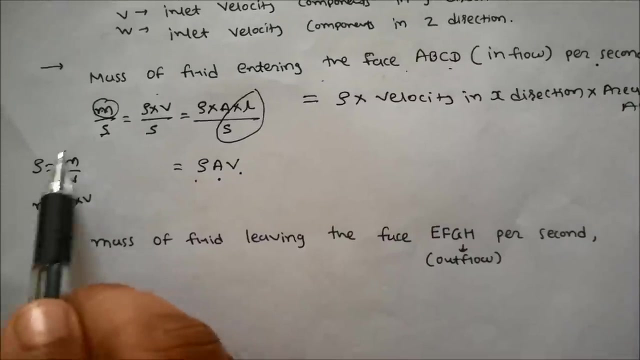 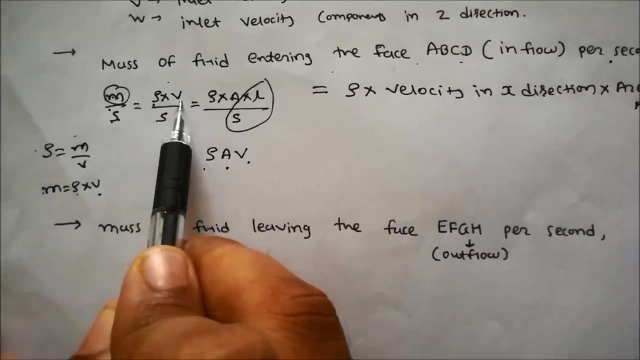 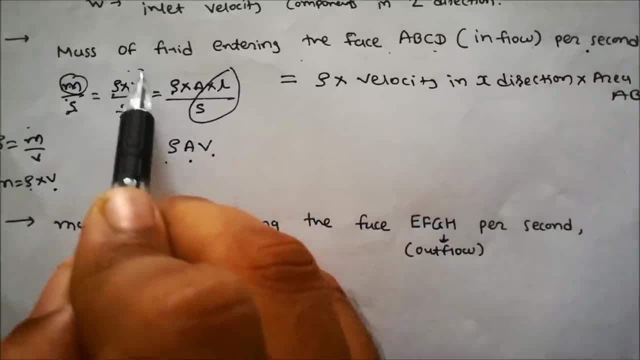 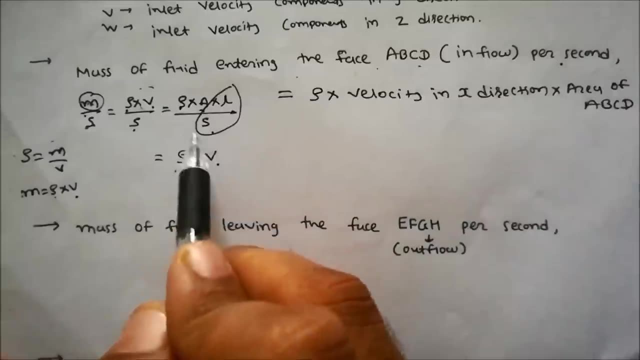 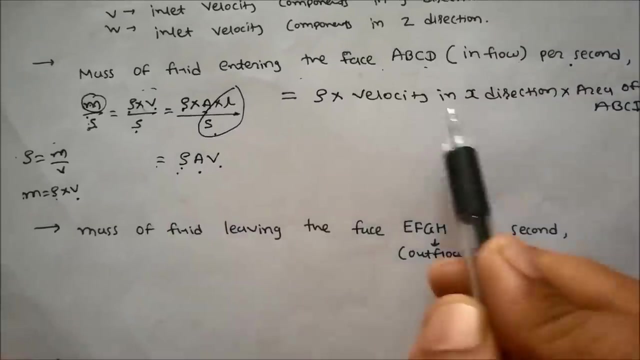 so density in place of volume. we can write area into distance, so a into l divided by second. so what is the meaning of distance per unit time? that is velocity. so final equation: mass per second is equal to density multiply velocity in x direction, multiply area of abcd. 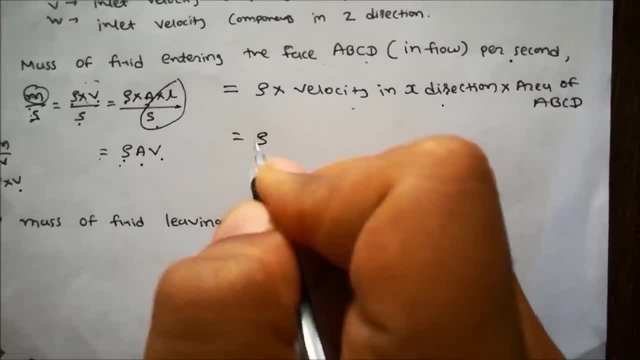 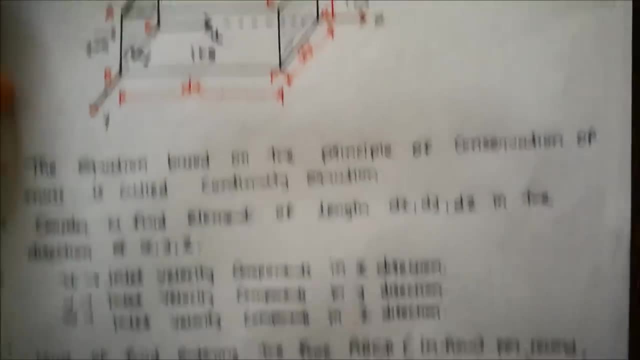 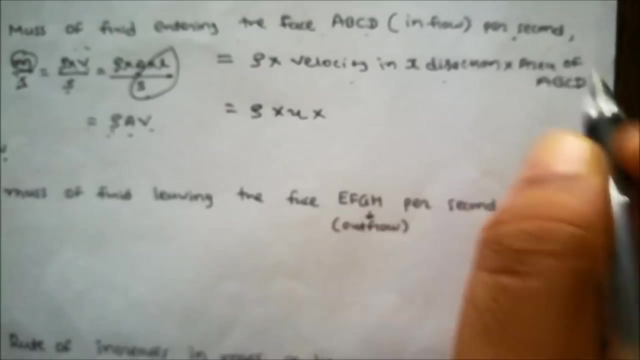 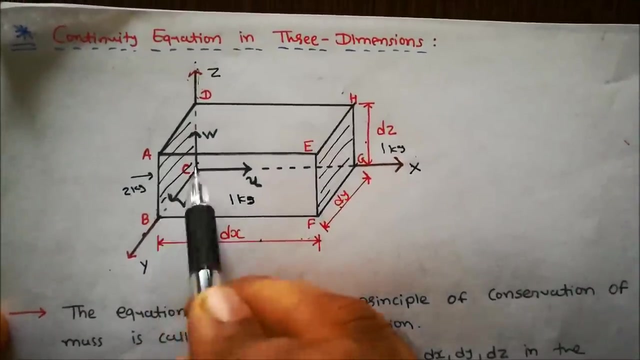 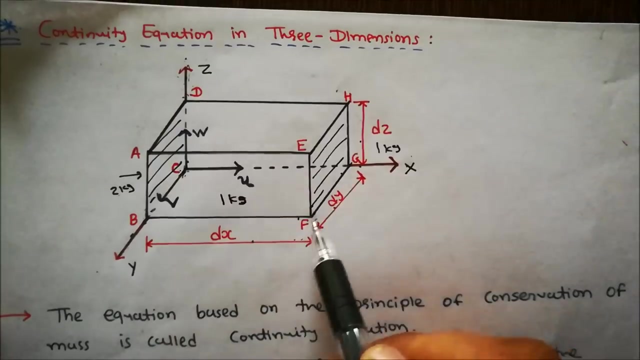 so rho. as it is velocity in x direction, that is component velocity. component in x direction, that is u. so velocity in x direction, we write rho multiply u, an area of abcd. area of abcd that we find here, area for abcd, so that is, length is dy and this length is dz, so area for abcd, that is. 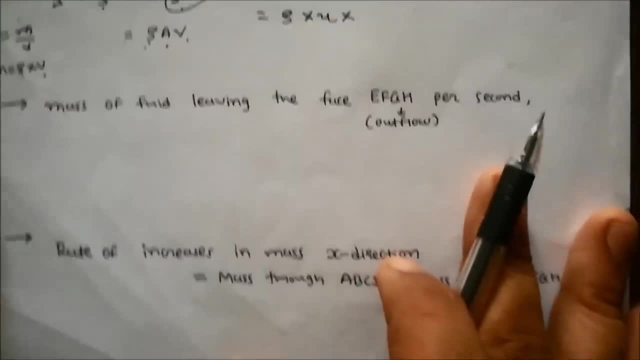 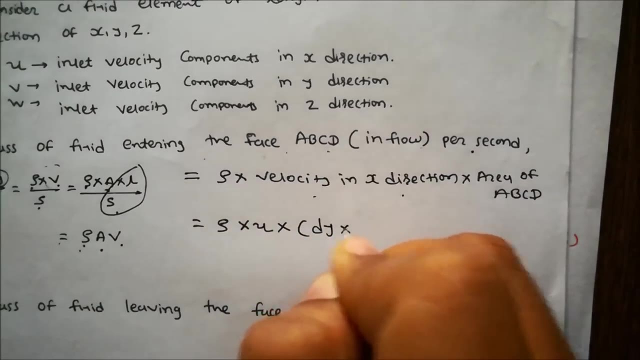 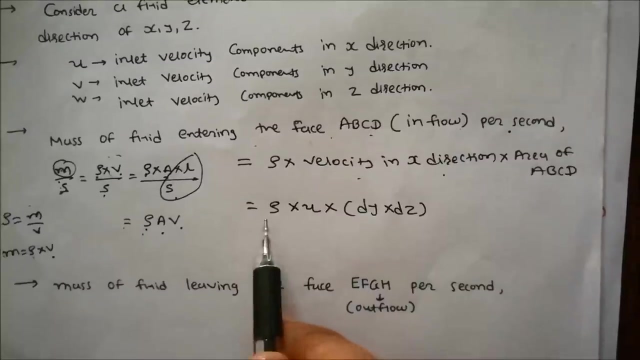 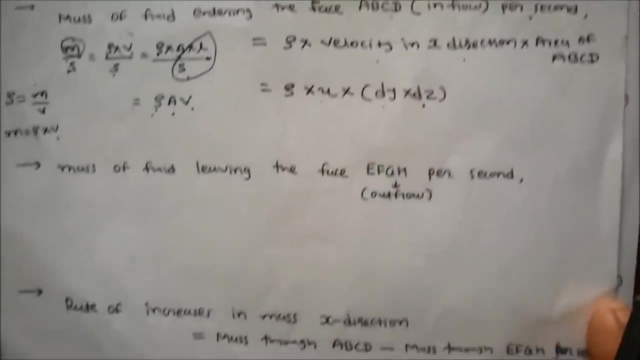 dy into dz. so in place of area we write area of abcd. that is dy into dz. so mass of fluid entering the phase abcd per second, that is rho u dy into this. Then we find mass of fluid leaving the face efgh per second. 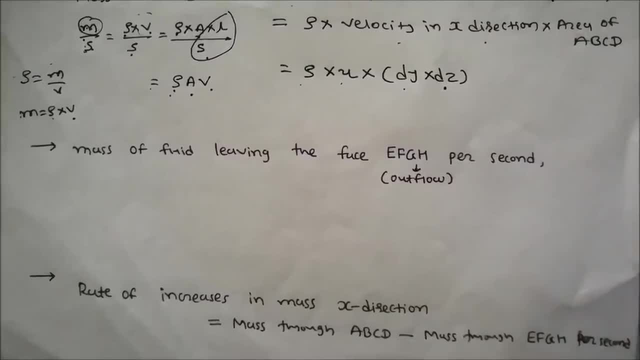 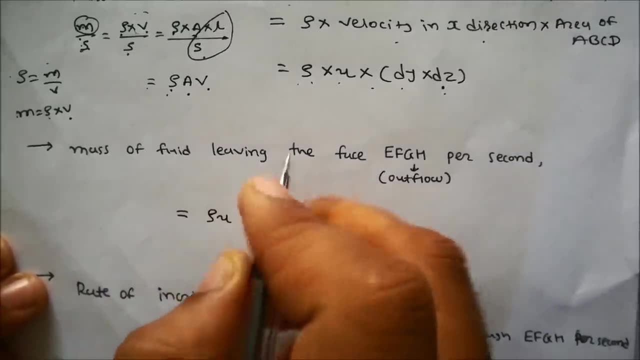 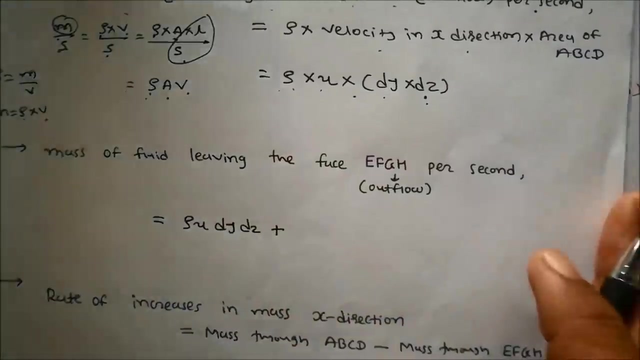 So first we write what is the mass entering the face abcd. that is, we find rho u dy dz. So first we write rho u dy into dz, Then if we here entering the mass, 2 kg and mass of fluid, leaving the face efgh, that is. 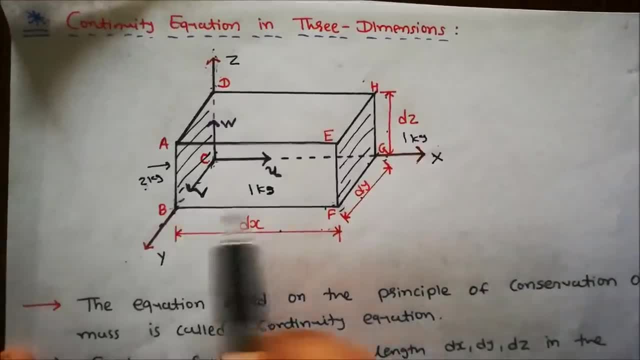 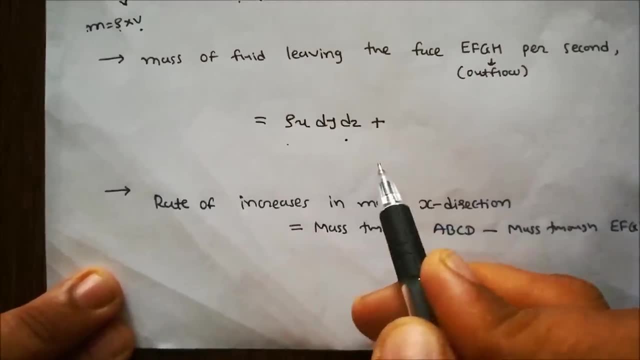 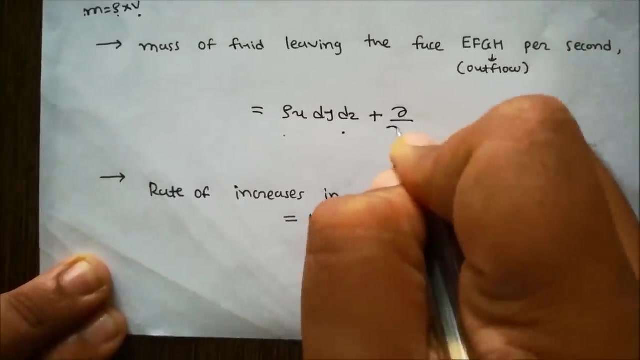 1 kg means with respect to distance, mass is changed. So here we write: first we write mass of fluid, entering the face abcd, then we find what is the change. So with respect to distance, mass is changed. So del by del x. here consider x direction. 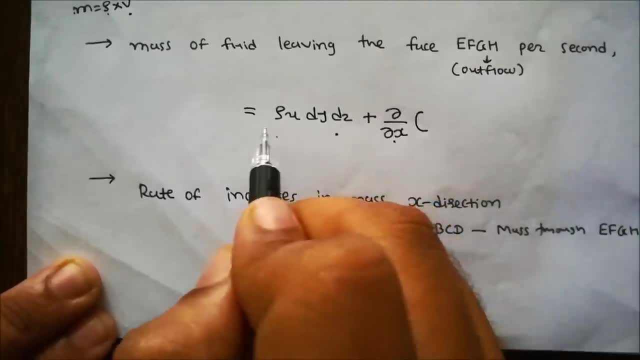 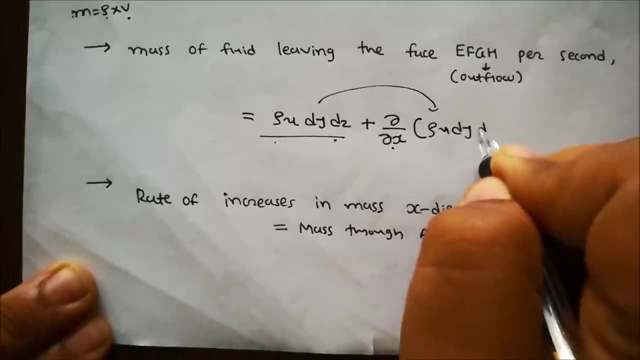 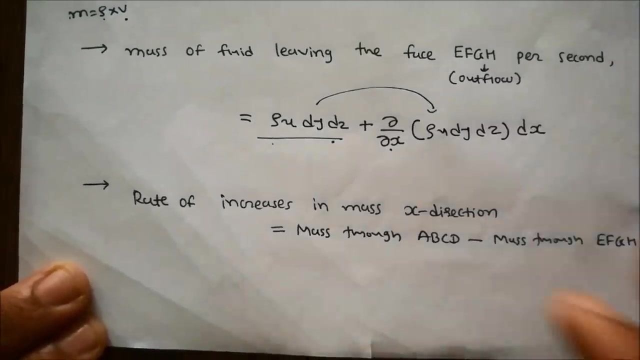 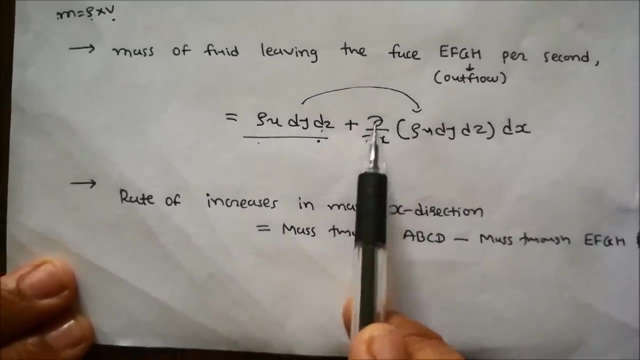 So del by del x. If we entering 2 kg mass, that means change is also in 2 kg mass. So del by del x. rho u dy dz into dx because of with respect to distance. So mass of fluid leaving the face efgh per second is equal to rho u dy dz plus del by. 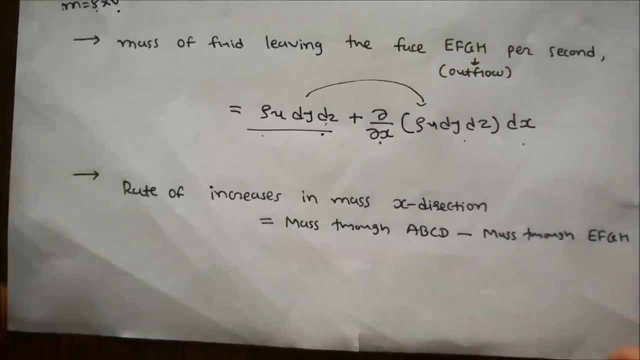 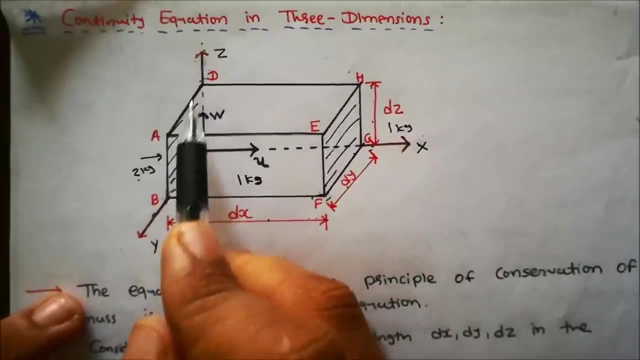 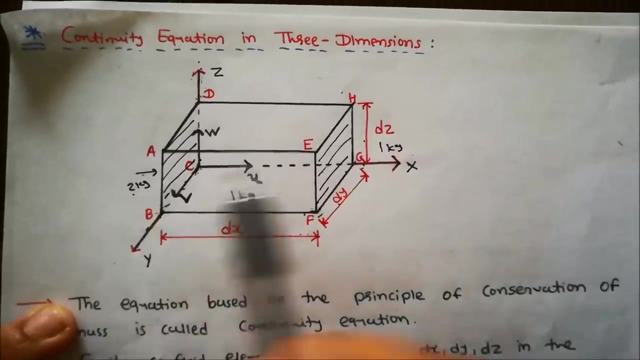 del x rho u dy dz into dx. So first we enter the mass Mass of fluid- abcd mass, abcd per second. So first we find mass of fluid entering the face- abcd per second, that is 2 kg. and then we find mass of fluid leaving the face efgh, that is 1 kg. 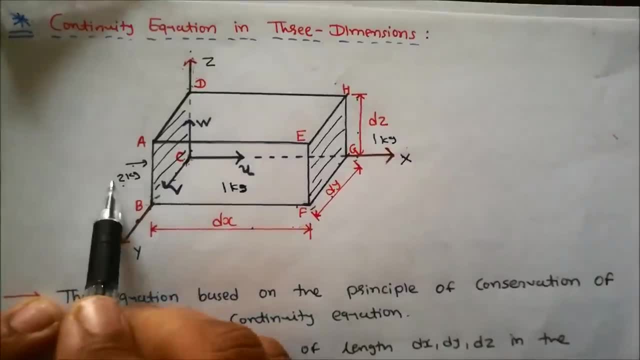 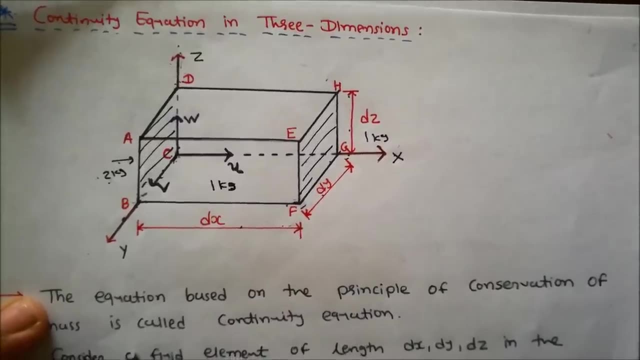 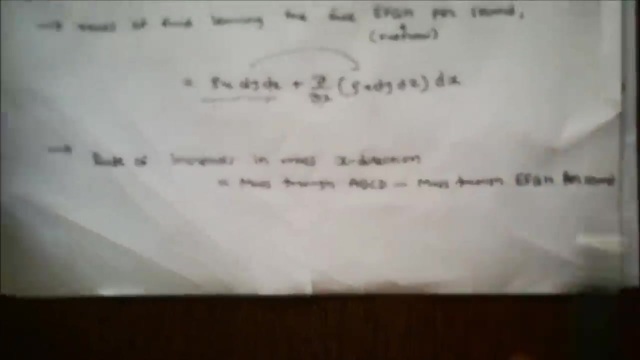 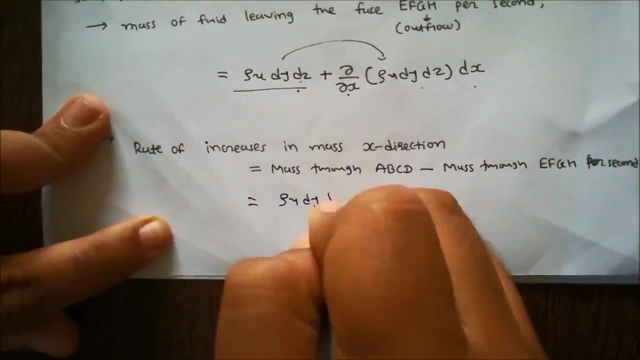 So what is the rate of increase in mass x direction? that is 2 minus 1.. So 1 kg. so we find rate of increase in mass in x direction that is mass through abcd minus mass through efgh per second. So here we write mass through abcd, that is rho u dy dz. 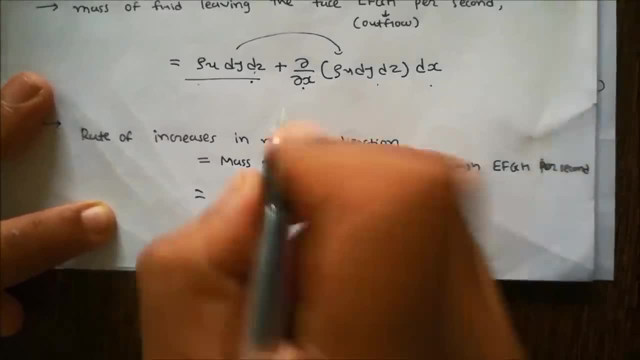 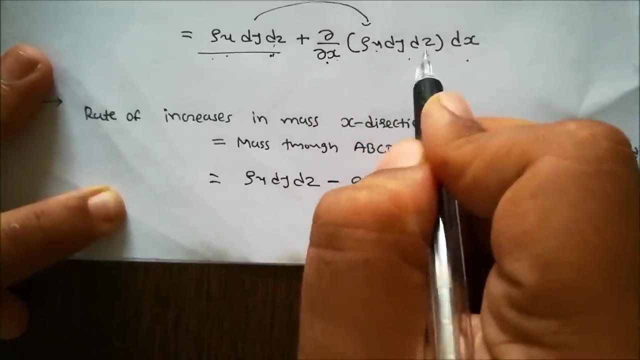 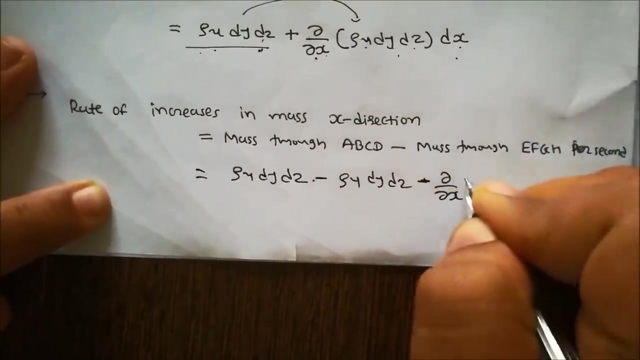 Minus mass through efgh per second. that is rho u dy dz plus del by del x. rho u dy dz dx, Here minus, so that is minus sign. So minus del by del x, Minus del by del x. rho u dy dz into dx. 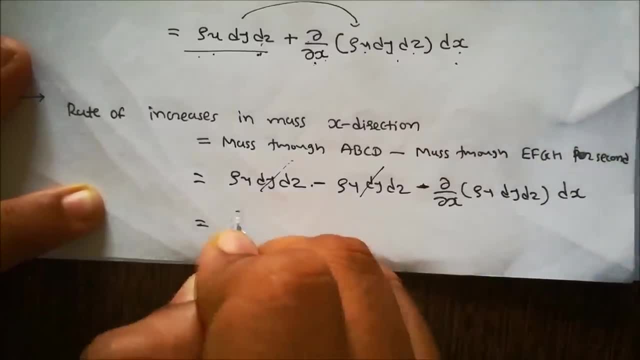 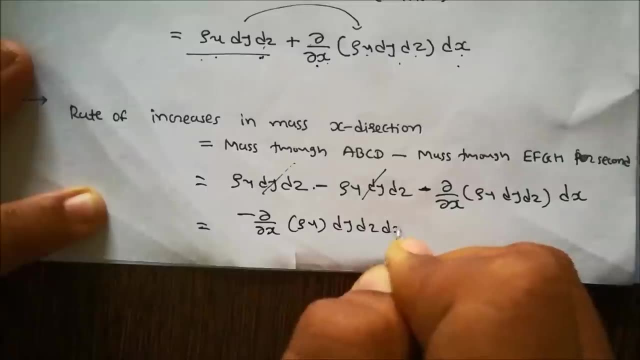 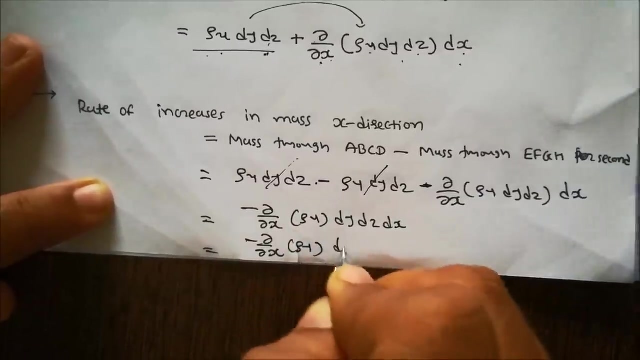 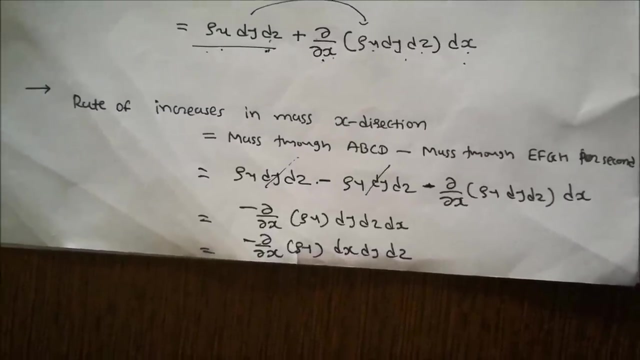 So rho u dy dz cancel out. So we get minus del by del x rho u dy dz into dx. So rewrite this equation: that is minus del by del x rho u dx dy dz. So in this way We find rate of increase in mass in x direction. 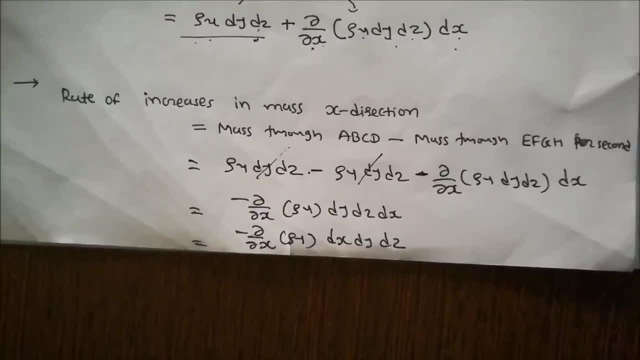 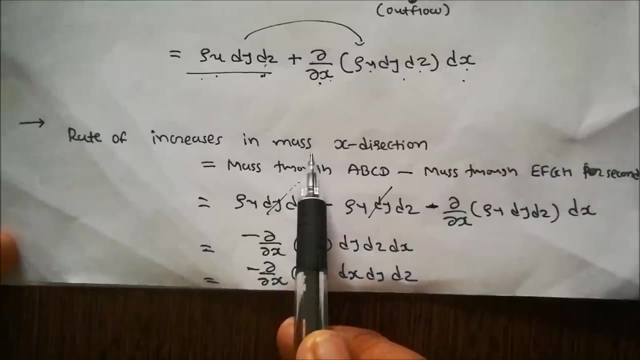 Here we consider 3 direction: x, y and z, because we find continuity equation in three diameter. So we find similarly rate of increase in mass y direction and rate of increase in mass z direction. So what is the rate of increase in mass x direction? 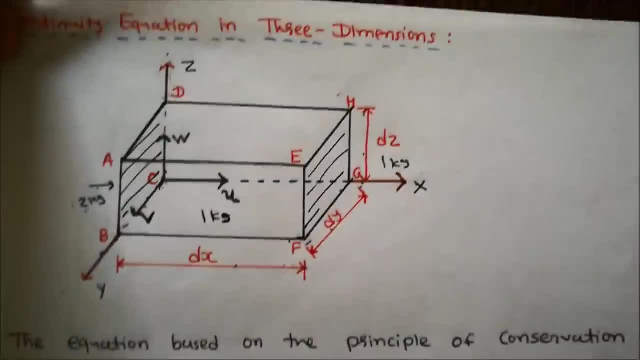 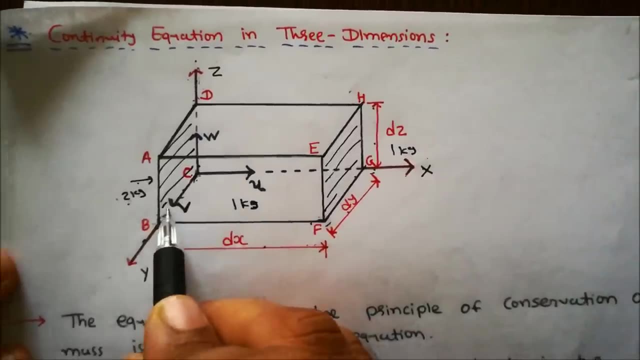 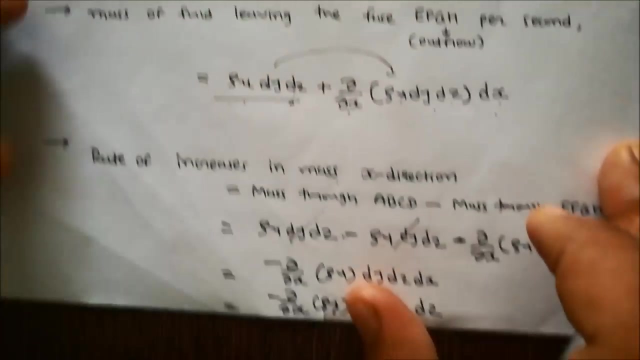 In place of u, here y velocity component, That is v. So when we find rate of increase in mass y direction, That is v, then take velocity component v, and if we find rate of increase in mass in z direction, then taken component w. so if we find rate of increase in mass y direction, then here minus del by: 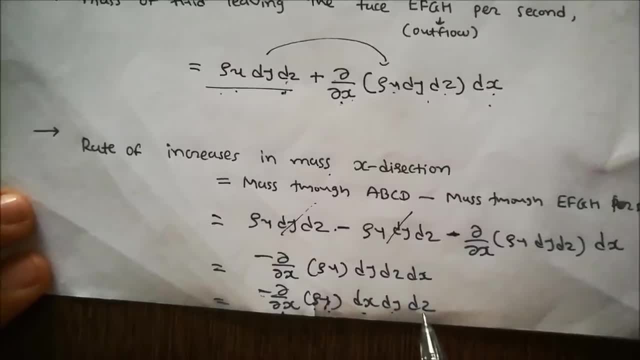 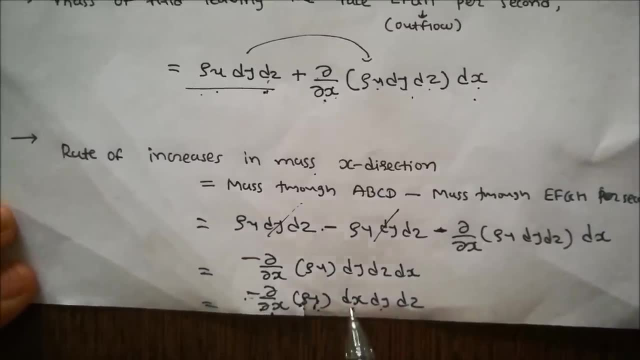 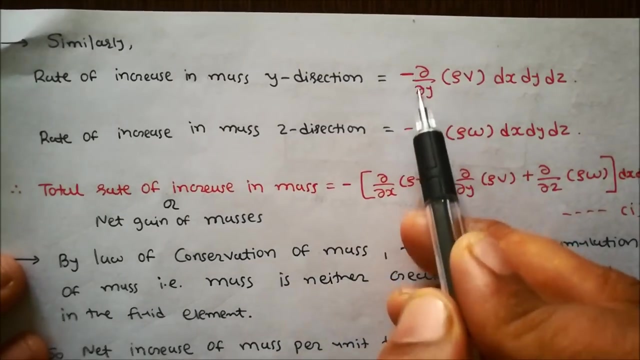 del y rho v dx dy dz. and if we find rate of increase in mass z direction that is minus del by del z rho w dx dy dz. so next we find rate of increase in mass y direction that is minus del by del y rho v dx dy dz. and then we find rate of increase in mass z direction. 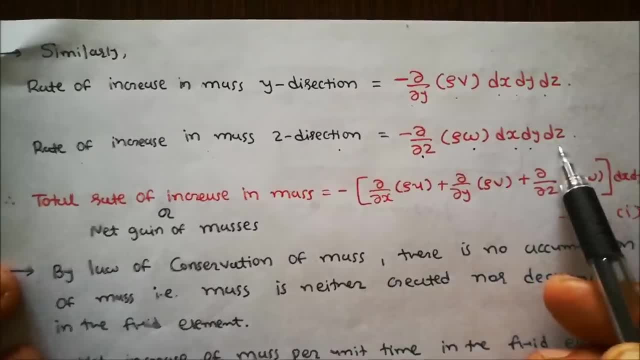 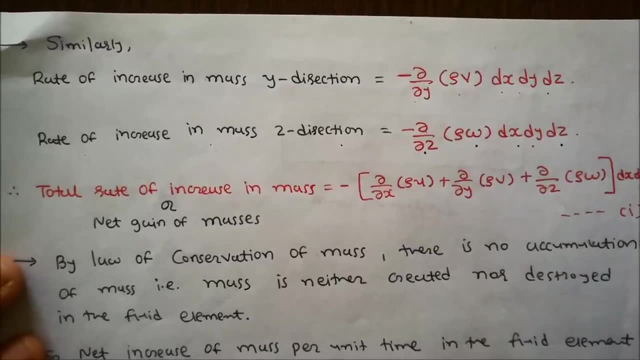 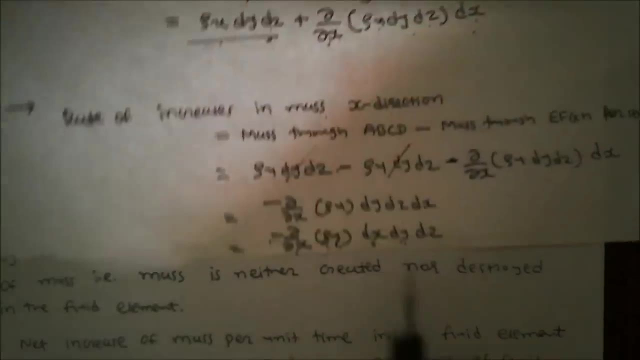 that is minus del by del z rho w dx dy dz. so what is the total rate of increase in mass? or you can say net gain of mass. that is the summation of these three direction. so minus common. So first we find x direction. so for x direction, del by del x rho u dx dy dz. so dx dy dz, common. 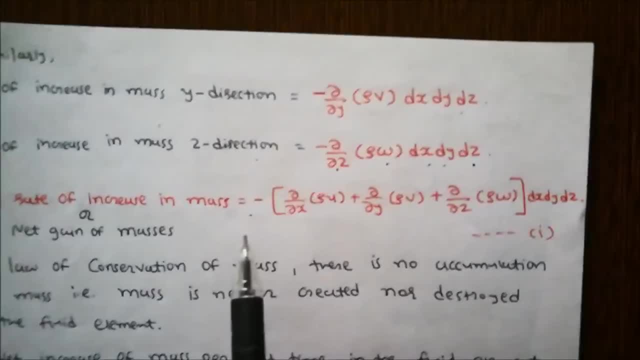 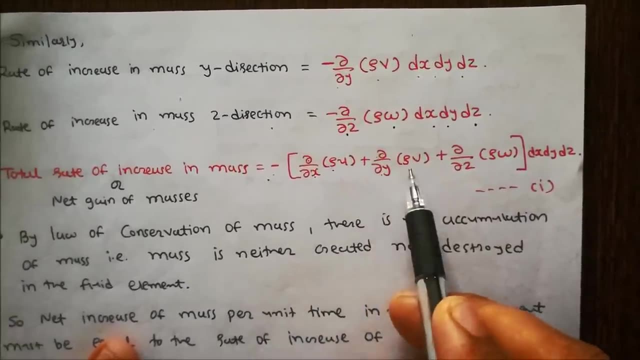 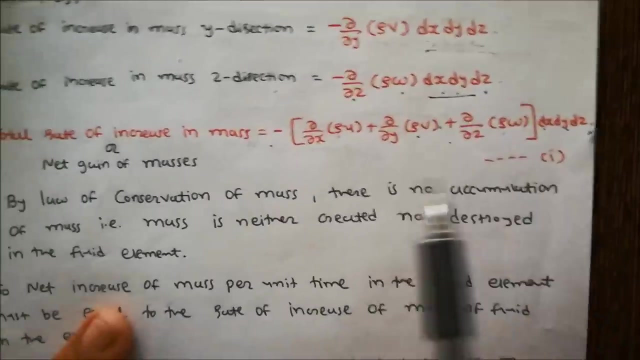 in all three direction. and minus common, so minus. we write common. minus v common so del by del x rho u plus del by del y rho v plus del by del z rho w and dx dy dz common so dx dy dz common So total rate of increase in mass. 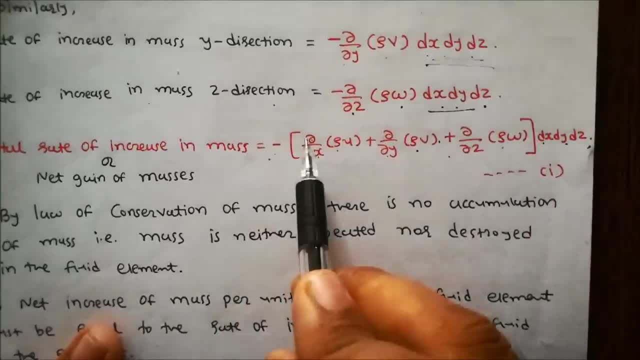 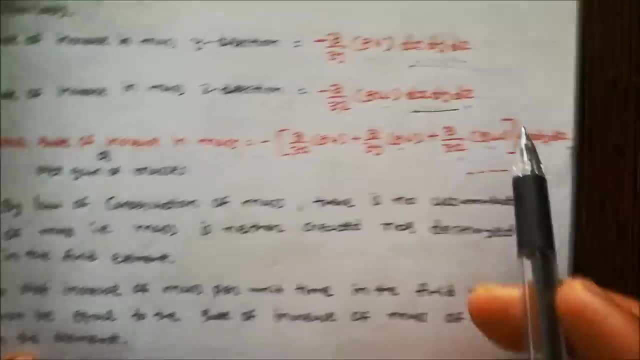 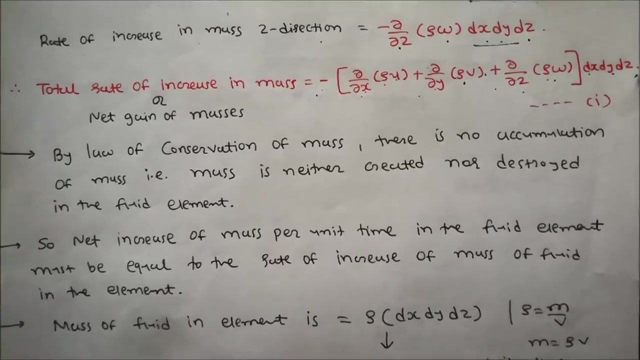 Or you can say net gain of mass. that is minus del by del x rho u, plus del by del y rho v, plus del by del z rho w, common dx, dy, dz. then continuity equation is based on the conservation of mass, that is, mass is neither created nor destroyed in the fluid element. 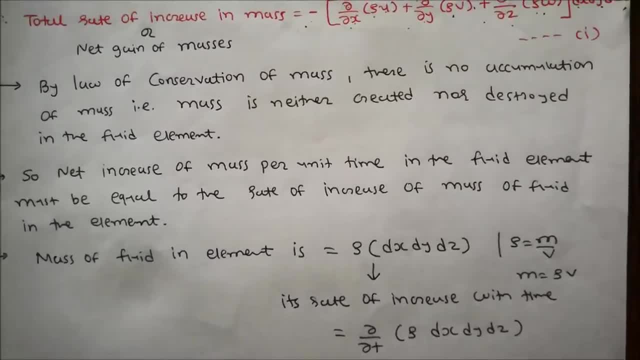 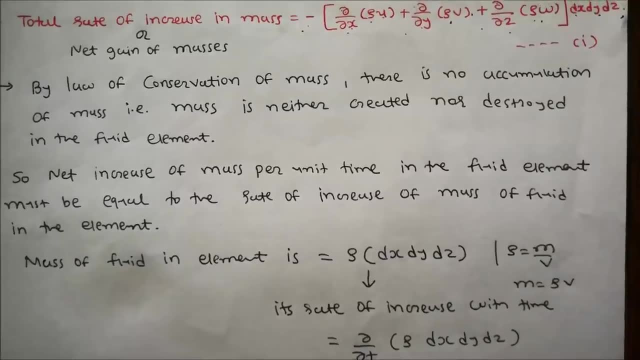 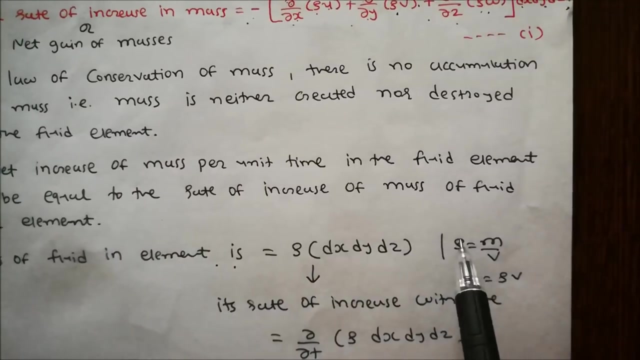 So net increase in net increase of mass per unit time in the fluid element must be equal to the. So the rate of increase of mass of fluid in the element. so mass of fluid in the element that is, we find if we know that density is equal to mass per unit volume. so mass is equal. 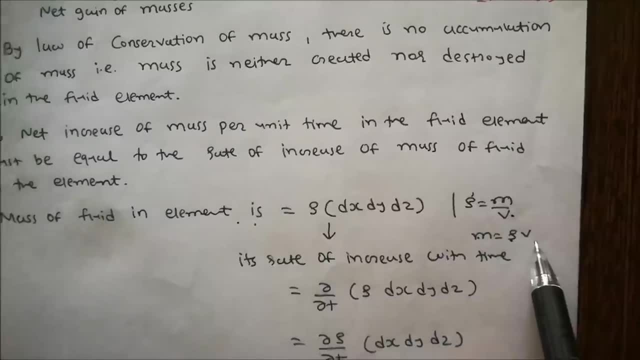 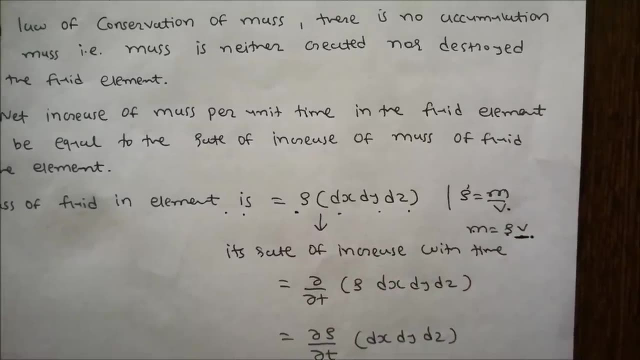 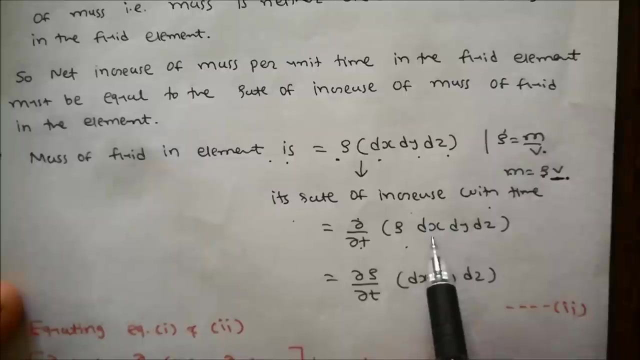 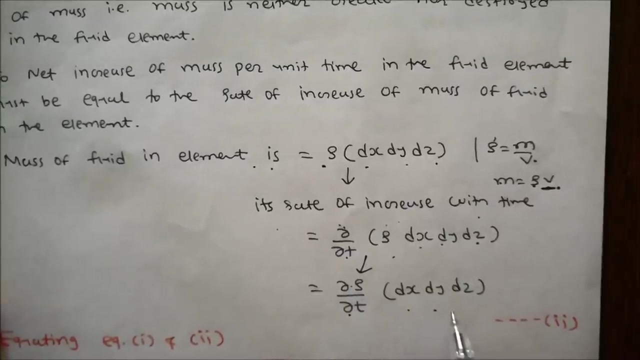 to density multiplied volume. so mass of fluid in the element is rho into dx, dy dz, because volume of the element, that is the dx into dy into dz, so it's the rate of increase with time. So We write this equation: so delta rho by delta t, dx, dy, dz. so this is the mass of fluid in. 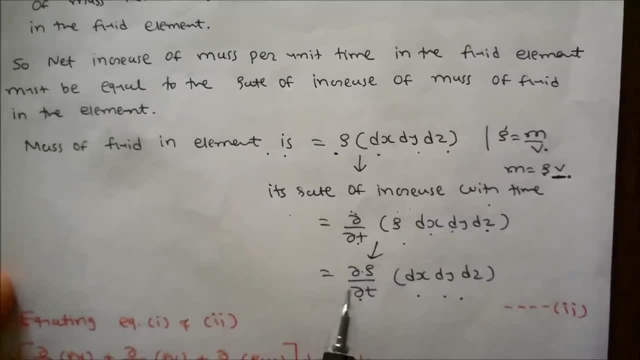 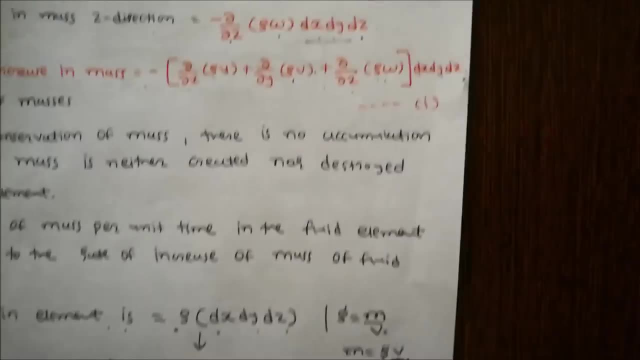 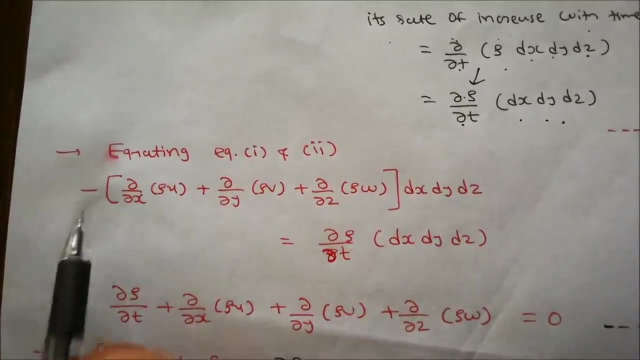 the element, and this mass of fluid of element must be equal to the total rate of increase in mass. so we compare equation number one and equation number two. equating equation number one and two, We write So: delta rho by delta t minus del by del x rho u plus del by del y rho v plus del by del.